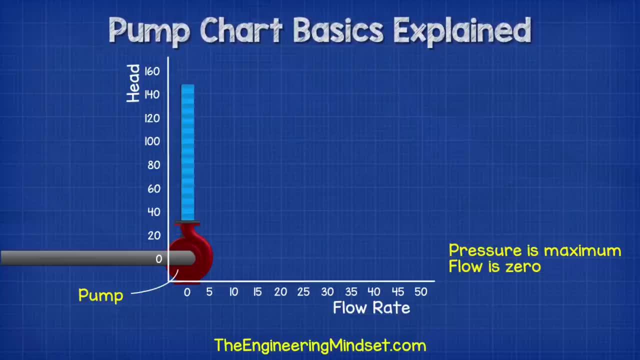 high as it possibly can within the pipe. At this point it's just spinning the same bit of water, which isn't good for the pump. so you don't want to run a pump like this in the real world. By recording the values during the elevation, we 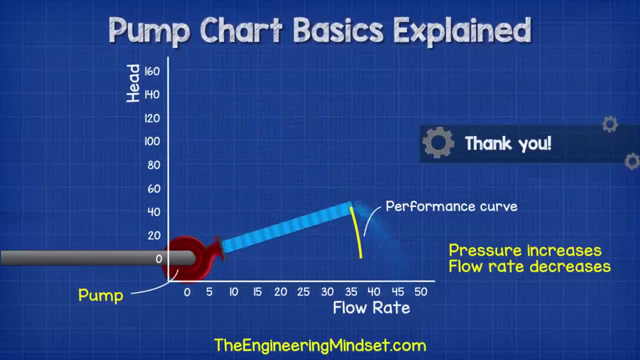 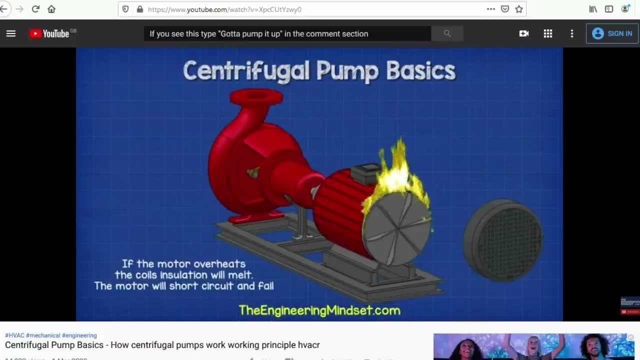 basically get our pump curve, although I will note, the pump manufacturers don't test pumps this way because it's just not practical. If you want to know how a centrifugal pump works, then we have covered this in detail in our previous video. Do check that out. links down below. 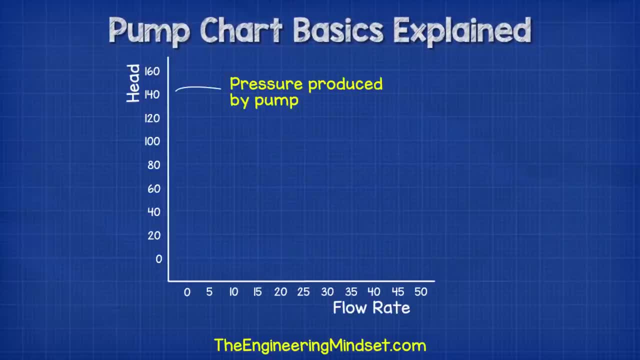 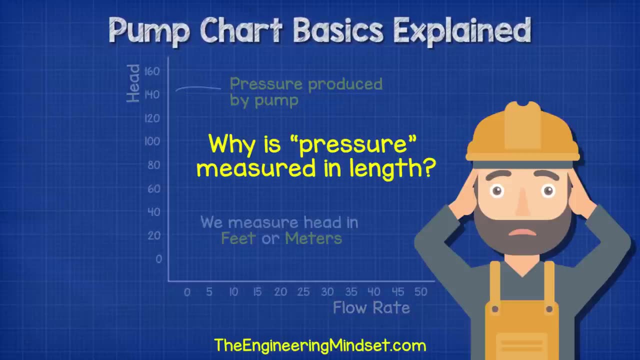 Head is shown on the vertical axis and this is referring to pressure, so we often hear the term head pressure. We measure head in feet or meters, which doesn't seem correct considering we're talking about pressure, Especially as you see the pressure gauges on the pump typically reading psi or bar. The reason: 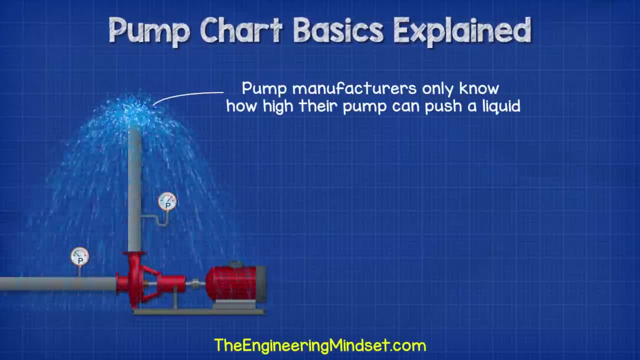 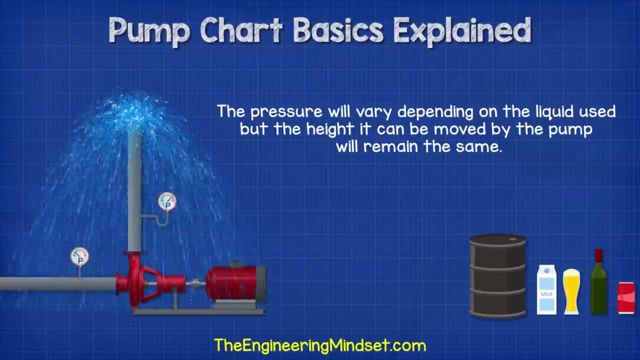 for feet or meters, is that pump manufacturers only know a how high their pump can push a liquid. They do not know which liquid your system will be pumping and, as each liquid has different properties, the pressure will vary depending on the liquid used. However, the height it can be. 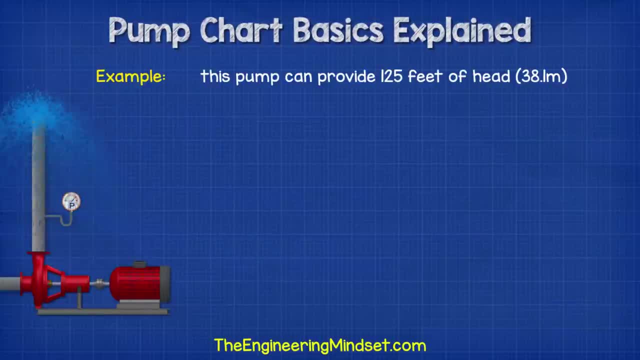 moved by the pump will remain the same. For example, we have this pump which can provide 125 feet of head. If we use it to pump water, the pressure will be around 54.25 psi, but if we were to use it to pump milk, then the pressure will be. 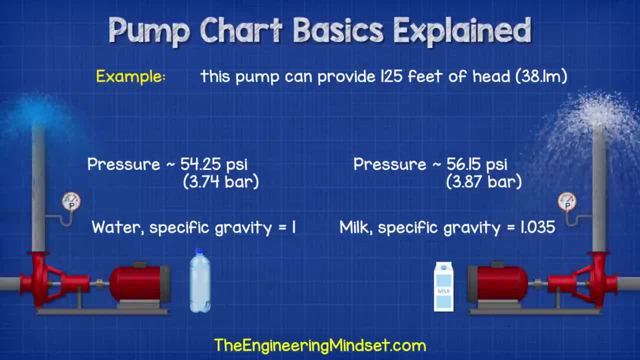 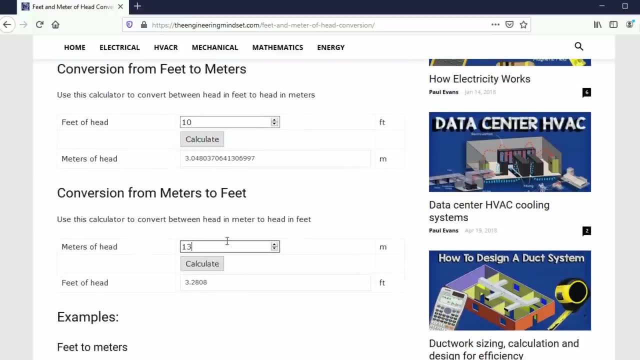 6.15 psi, and that's purely because of the properties of the two fluids. Conversion between feet and meters of head is very easy. We have a free calculator for that, which you can find links to in the video description below. Why do we need to know head pressure? Pumps are usually used to move liquid to. 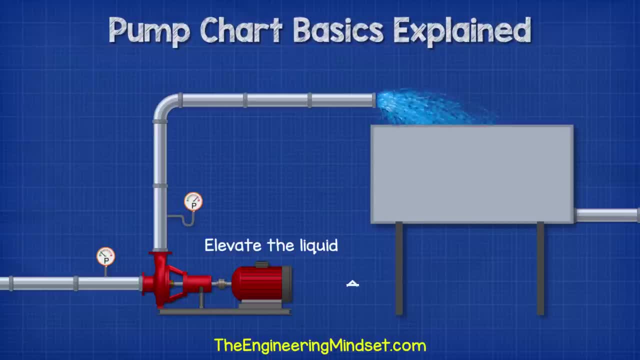 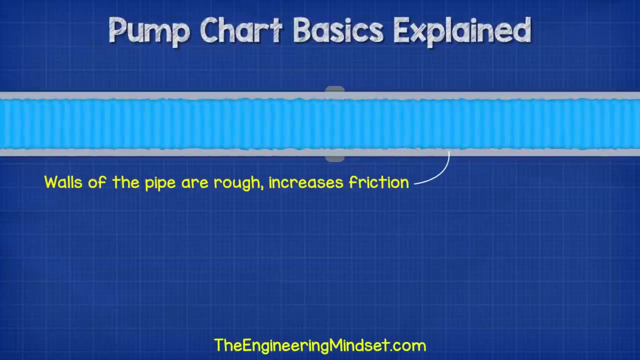 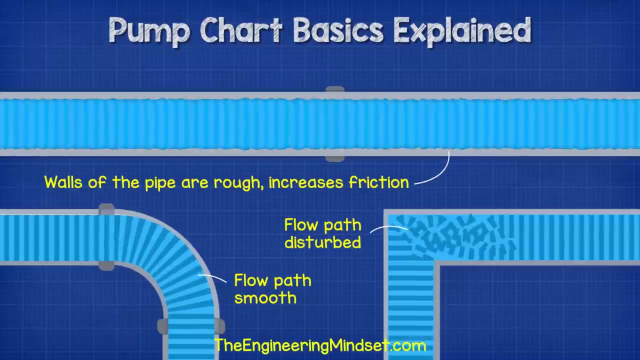 a higher region, so we need to ensure the pump can reach this elevation. As we pump liquid through the pipes and the fittings, friction will try to oppose the flow. This occurs from the walls of the pipe, but also disturbances to the flow. this causes pressure losses which waste energy from the pump. The amount of 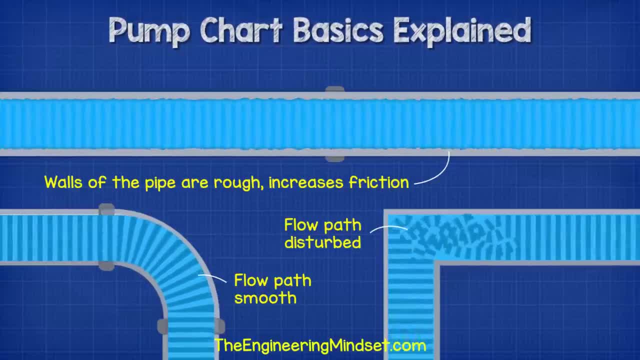 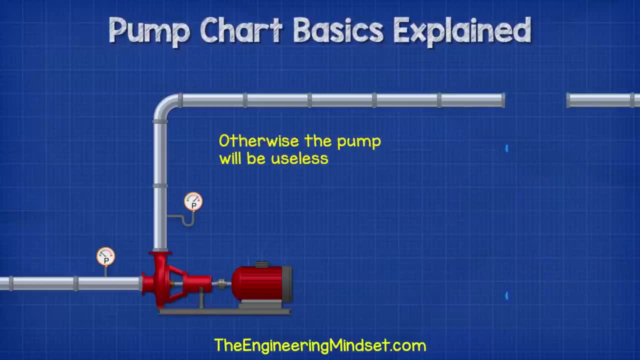 friction depends on the liquid type, as well as the materials and fittings used. Therefore, we must calculate how much friction or pressure loss our system will generate and ensure that the pump we select can overcome this. Otherwise, we're not going to get any liquid out the upper end When we look at the pump. 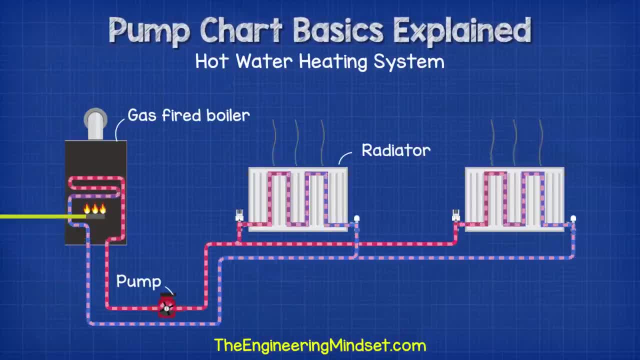 charts, we'll find pumps ranging in head and flow rate. For example, when we look at a small domestic heating system, there are a few fittings and short pipes. therefore, we can't get the pump to reach that level. We need to know how much room it needs to have to get into the pressure system. This causes pressure. 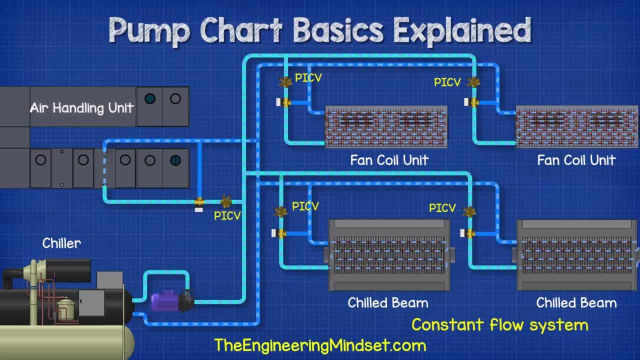 losses which waste energy from the pump. The amount of friction depends on the liquid type as well as the materials and fittings used. Therefore, we must calculate how much we would use a pump with a relatively low head pressure. But if we were to look at a commercial heating system, 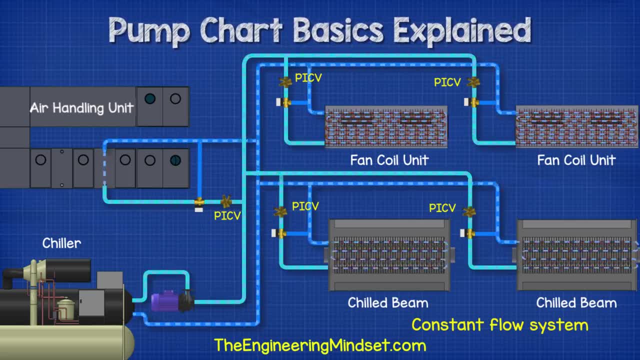 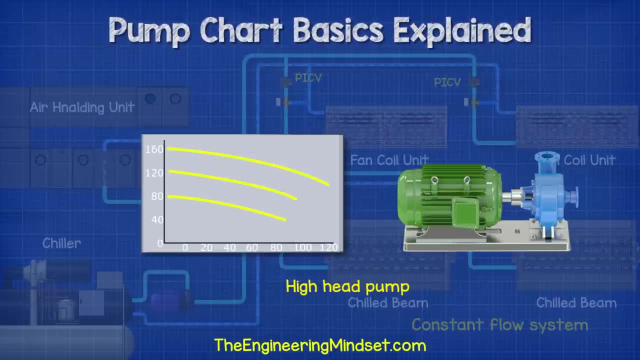 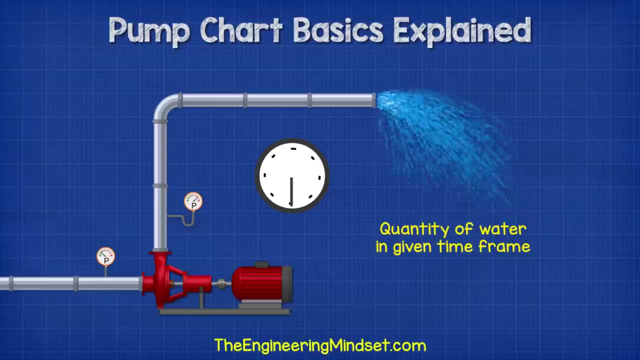 with multiple air handling units, fan coils and long pipe lengths, then we know the pressure drop will be much higher, so we would need a pump that can provide much more head pressure. The flow rate is a measurement of how much liquid is flowing from the pump in a given amount of time. 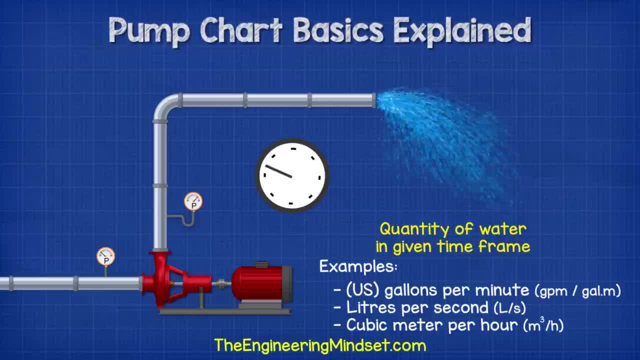 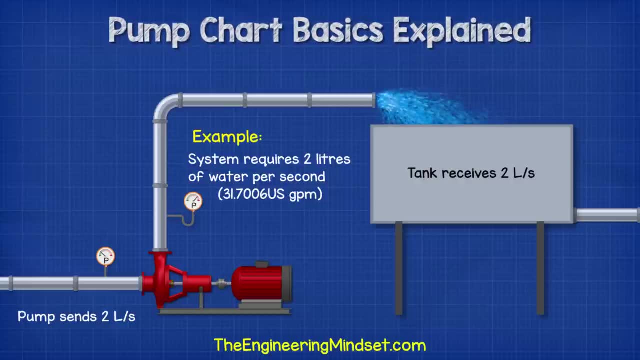 This measurement comes in many different units, for example gallons per minute, liters per second or cubic meters per hour. For example, a system might be designed to move two liters of water per second from a holding tank to a process tank. Performance curve. 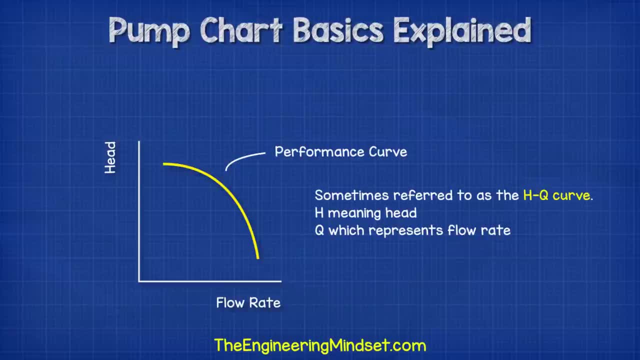 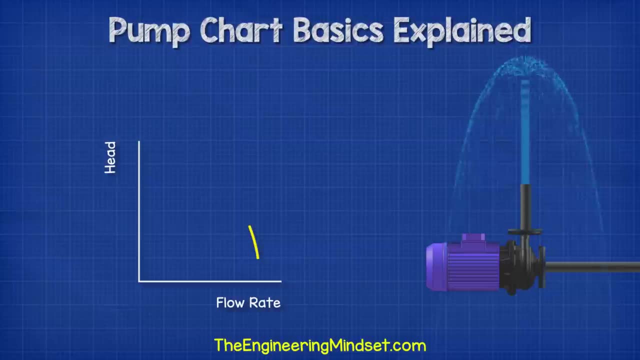 This is sometimes referred to as the HQ curve: H, meaning head, and Q, which represents flow rate. The manufacturer will test each pump to obtain the performance data and then plot this on the graph. This will represent all the possible configurations between flow rate and head pressure. 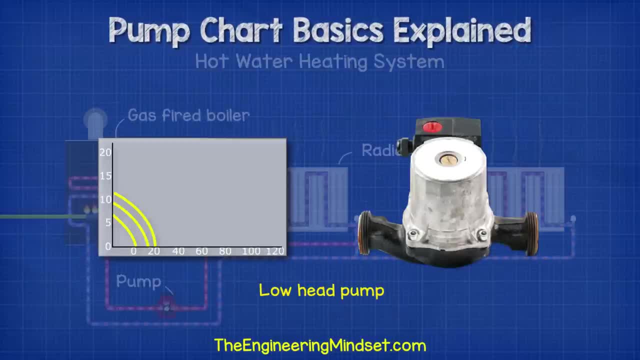 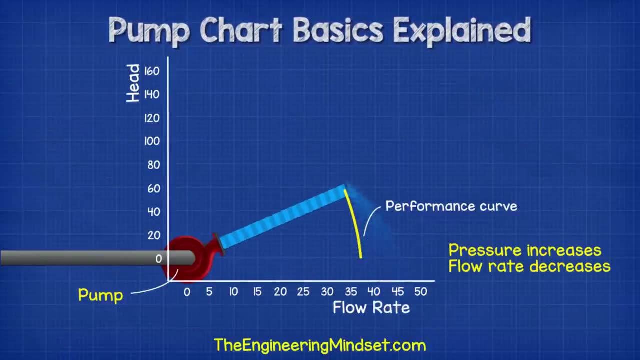 and we use this to check whether a pump will suit our requirements. The performance curve will be different for each pump and some will suit our system needs better than others. You will usually see that as the pump flow rate increases, the head pressure decreases. 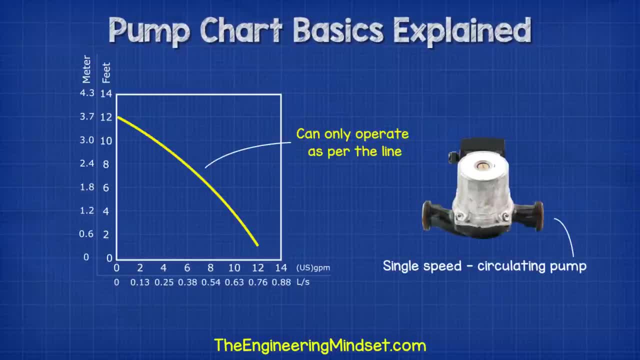 When selecting a circulating pump, the pump will only perform as per the line. So for this model, if we wanted eight gallons per minute, then we would have six foot of head. You can also get multi-speed circulating pumps, which we'll look at later on. 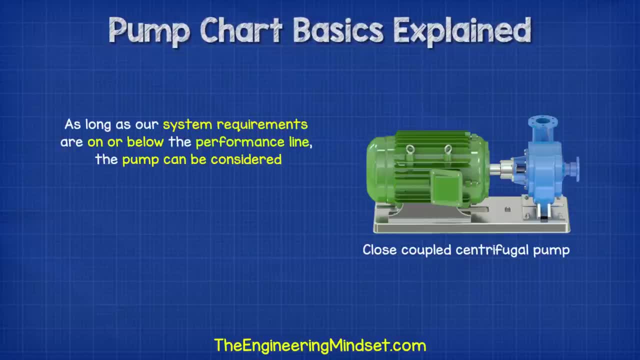 in this video. When selecting a larger centrifugal pump, as long as our system requirements are on or below the performance line, then the pump can be considered. We can potentially use a smaller impeller or variable frequency drive to better suit our requirements and again we're going to look at that. 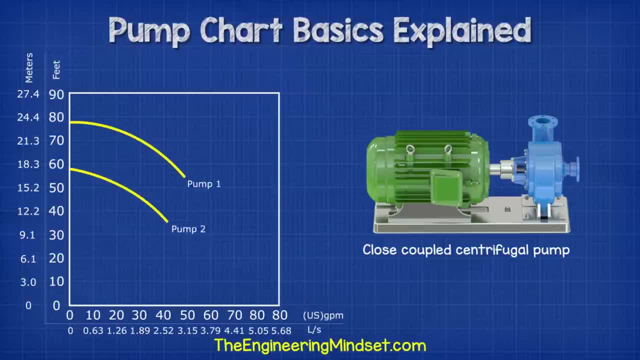 a little later. in this video, For example, the performance curve of two large centrifugal pumps are plotted here. We need a flow rate of 30 gallons per minute and a head pressure of 70 feet. That means that pump two can't be used. 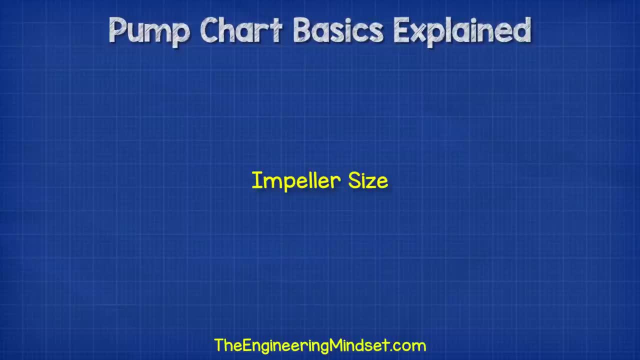 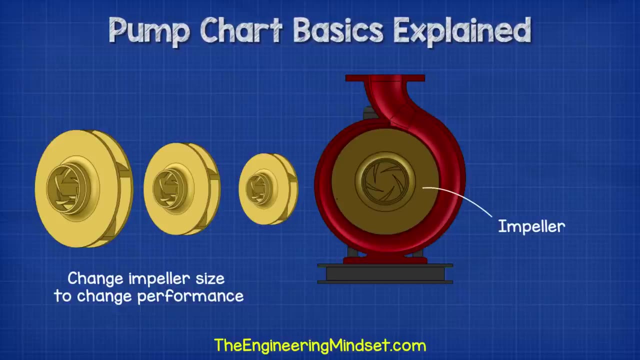 but pump one could be Impeller size. With centrifugal pumps we can often change the size of the impeller. The diameter of the impeller will change how much water can be moved. So on some charts you'll see multiple performance curves. 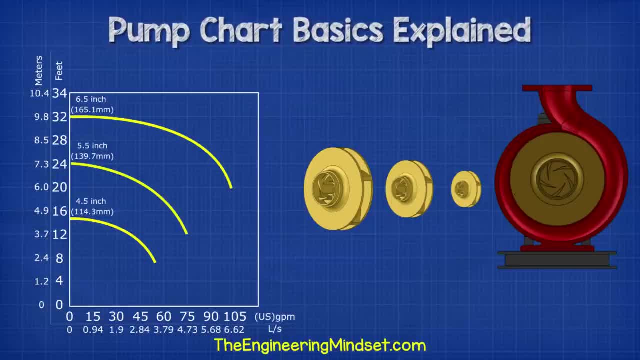 which will give us the performance details of the pump for different diameter impellers. For example, 30 gallons per minute for a 4.5 inch impeller gives us around 13 feet of head, But if we use the 5.5 inch impeller, 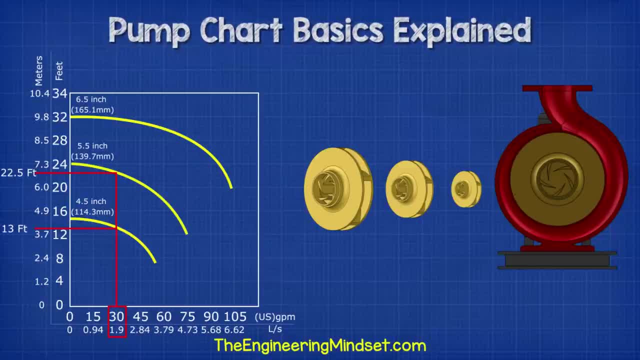 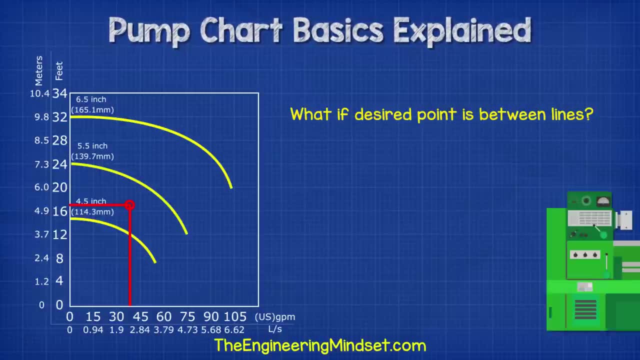 then we would get around 22.5 feet of head. In some instances our required flow rate and head pressure might fall between the two impeller diameter lines. In such cases we can often machine the impeller down to the required size to get a better match. 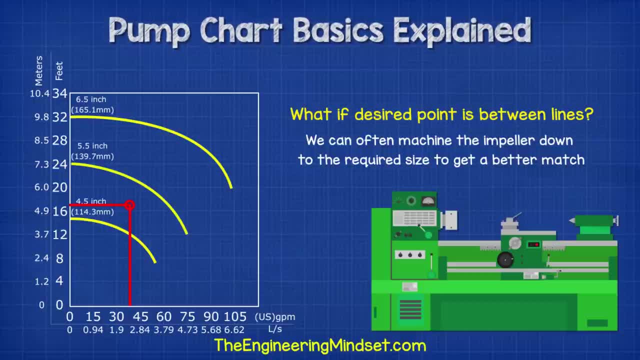 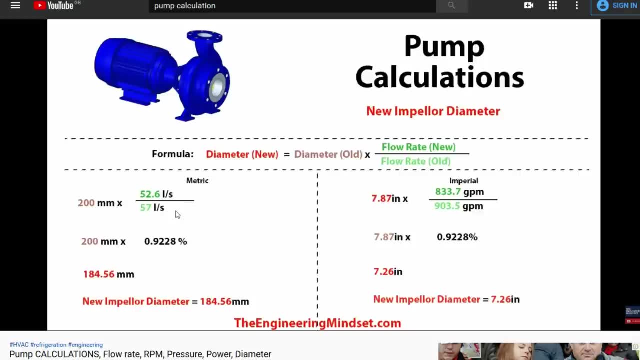 You should ask your pump manufacturer or pump specialist to carry out this service, though The performance of the pump will then need to be calculated. I'll leave some links in the video description below for worked examples for that Pump power. As we know, pumps require mechanical power. 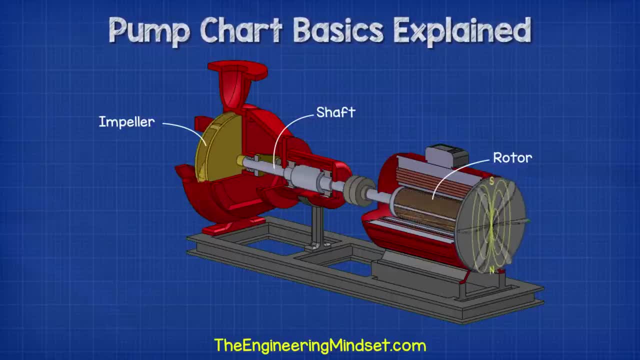 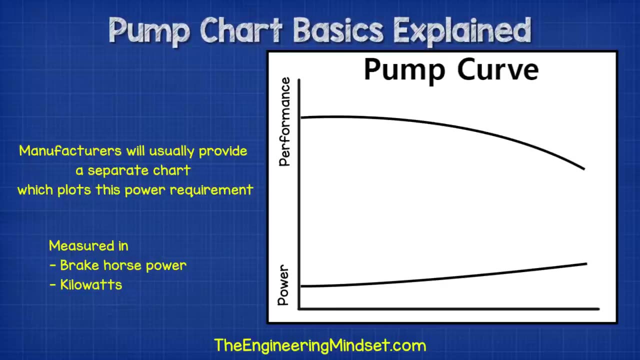 to spin the shaft rotor and ultimately move the water Pump. manufacturers will usually provide a chart which plots the power requirement. In imperial units we use brake horsepower and in the metric system we use kilowatts. With this chart we see the brake horsepower. 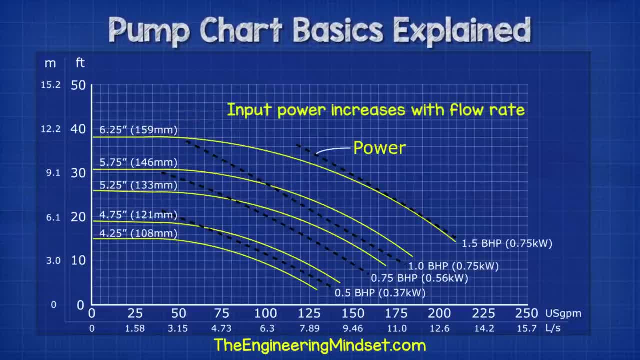 plotted at various intervals. As you can see, as the flow rate increases, so does the power requirement. We use this chart to size our motor. For example, if we needed 125 volts, if we needed 125 gallons per minute with 18 feet of head. 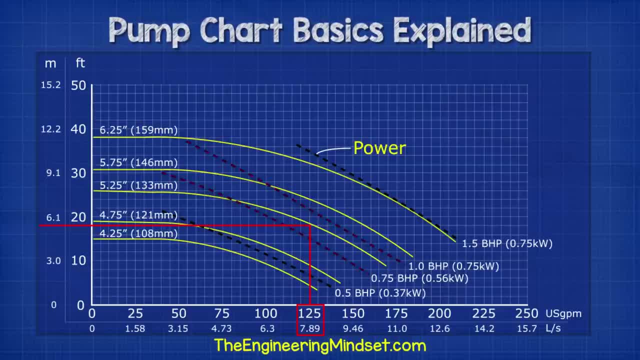 then this is between the 0.75 and the one horsepower lines. As this point is above the 0.75 line, this means we can't use a motor of this rating because it will not be able to cope. Therefore, we'll have to use a one brake horsepower motor. 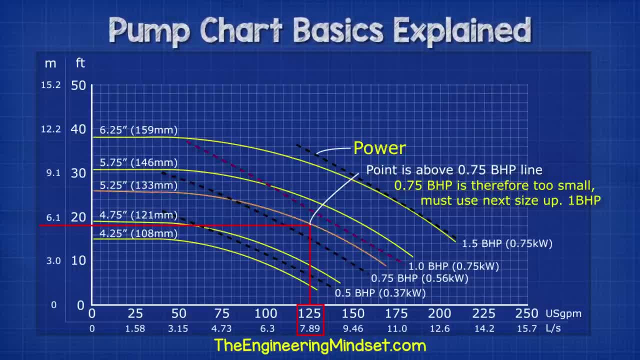 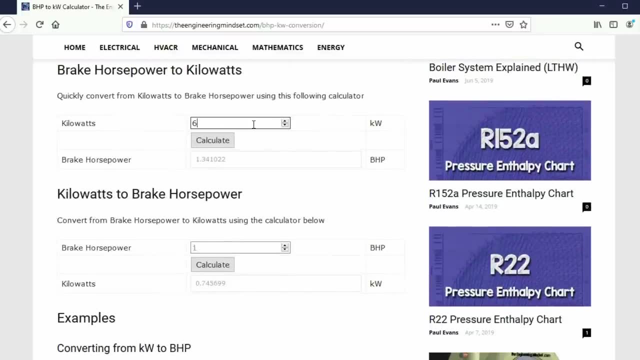 and we see the performance curve falls completely under this line. So if our head pressure calculation is wrong, then we do have some safety margin. If you want to convert between the two, between brake horsepower and kilowatts, then check out our free calculator. 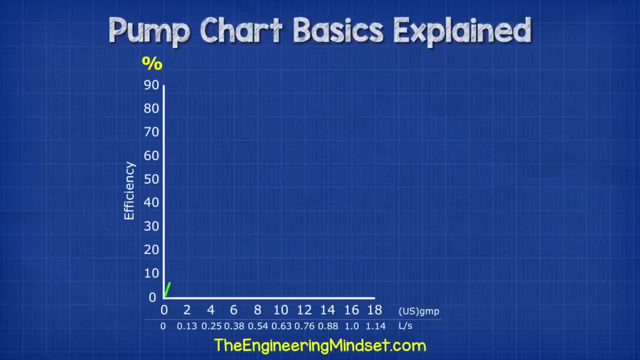 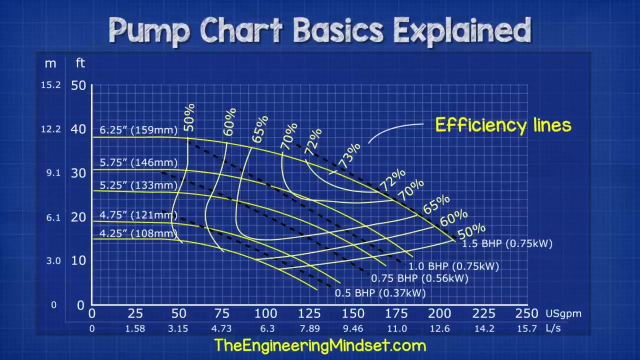 links down below. for that Efficiency. Some charts will display the efficiency curve of the pump. This is measured in percent. We'll usually see this curve line where the pump increases up to its maximum efficiency and then it starts to decline again. Charts that display different impeller sizes. 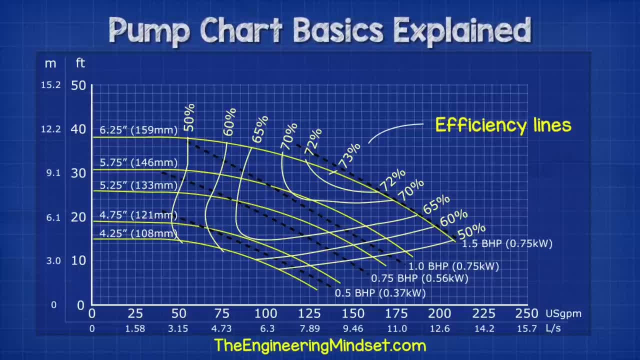 will usually have efficiency displayed in these more complex plot lines. Each line displays the percentage of efficiency In both charts. you can see that the efficiency varies depending on how you operate the pump. In multiple impeller size charts we see that the efficiency decreases. 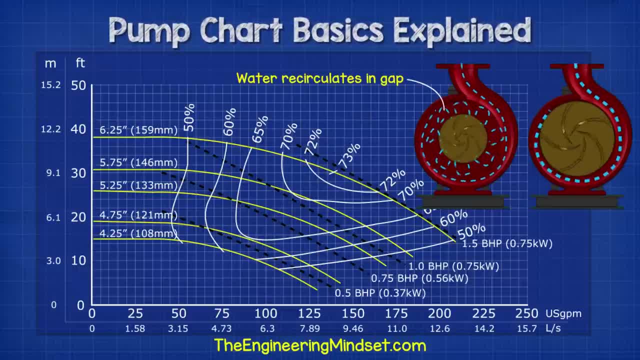 as the impeller size also decreases and that's because the gap between the impeller and the pump casing increases, and that will allow water to recirculate in this region and therefore waste energy. The efficiency is the ratio or comparison between the amount of energy going into the pump. 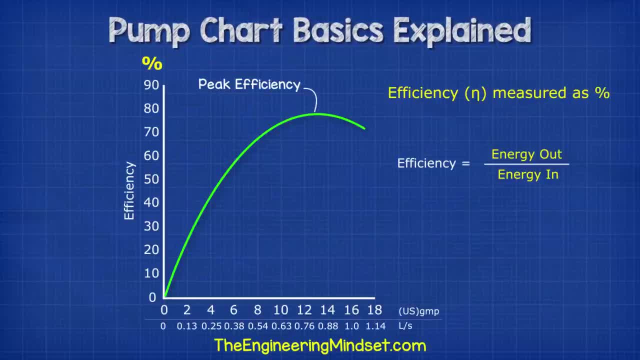 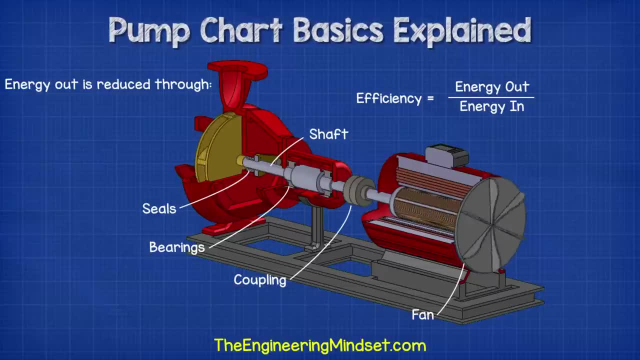 versus the amount of energy we get out of the pump. So ideally we want this to be as close as possible to the peak for optimal performance. The pump will always lose some power when it converts and transmits this electrical energy into mechanical energy. 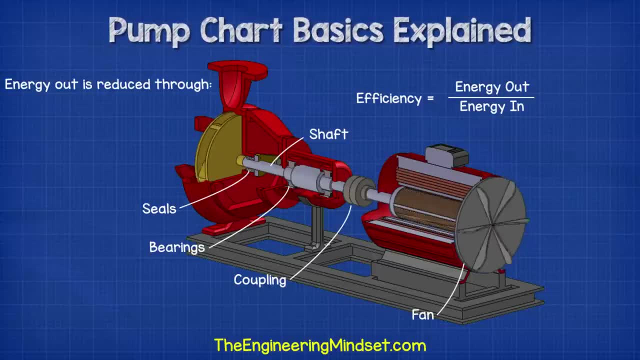 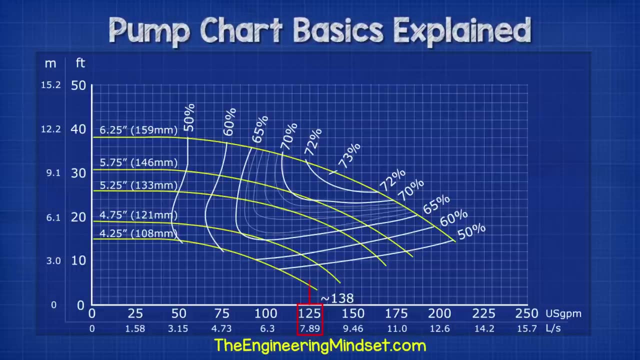 and this will be lost through the couplings, the bearings, the shaft, the seals, the cooling fan, et cetera. For example, on this chart we can see that if the pump provided 125 gallons per minute at 25 feet of head. 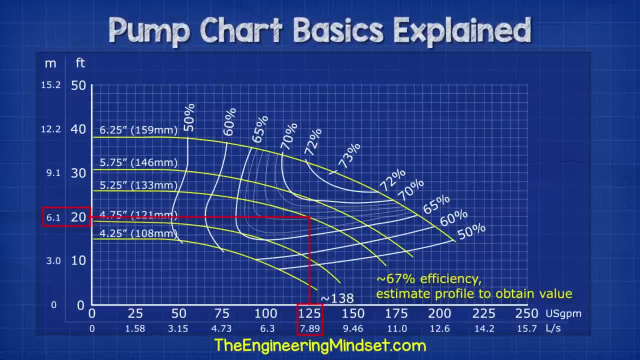 then it would run at around 67% efficiency, which isn't very good. If the same pump operated at 30 feet of head for 138 gallons per minute, then it would operate at its peak performance of 73%, which is much better. 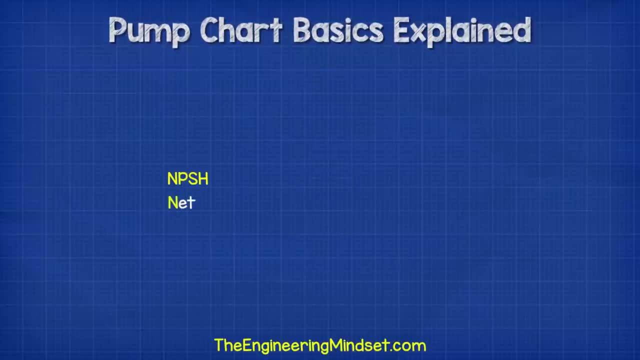 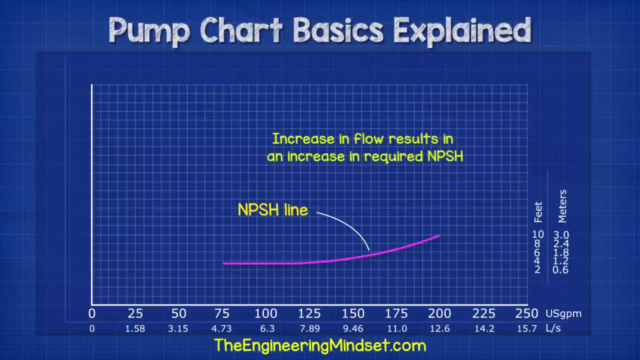 MPSH. this is the required MPSH or net positive suction head pressure. This usually has an upward curve, which means as the pump flow rate increases, we see the MPSH value also increases. We measure this in meters or feet, sometimes kilopascals. 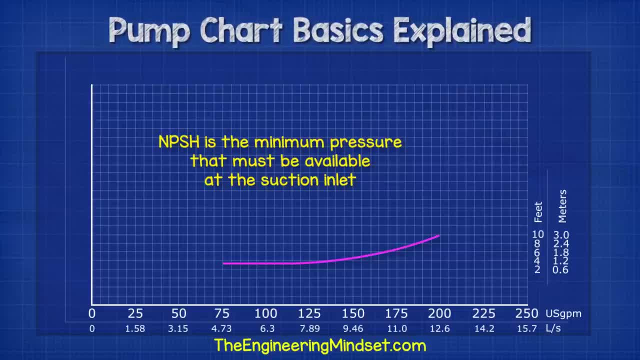 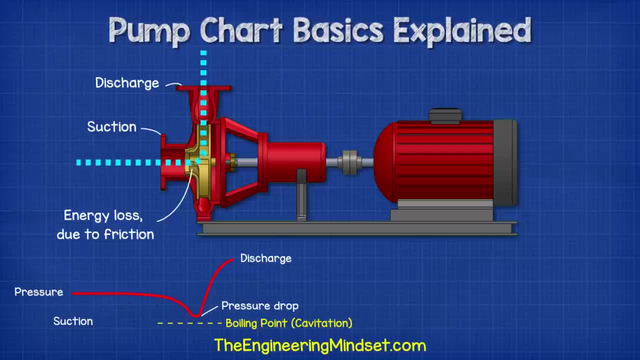 The MPSH is the minimum pressure that must be available at the suction inlet of the pump to overcome the entrance losses and avoid cavitation. The available pressure at the inlet must therefore be greater than this value. Pump cavitation is where the pressure at the inlet of the pump reaches a low enough point. 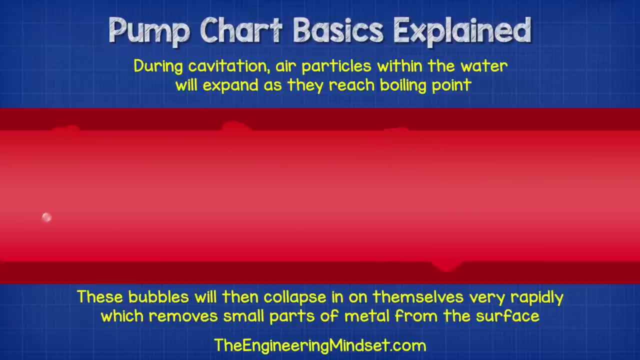 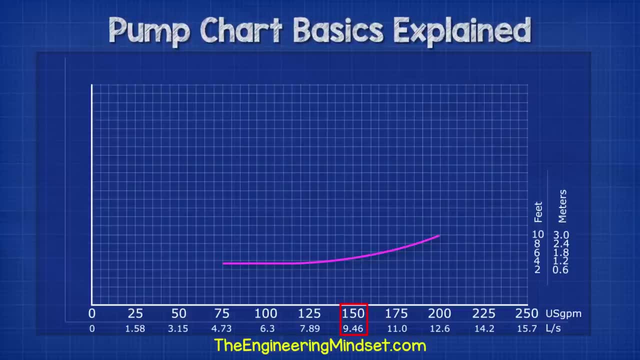 that the water begins to boil. This creates rapidly expanding and collapsing air bubbles, which will gradually destroy the surface of the pump and the casing. For this example, if we were to move 150 gallons per minute, then we would require an MPSH value. 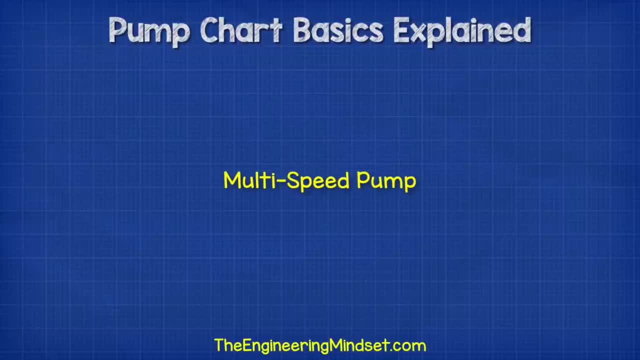 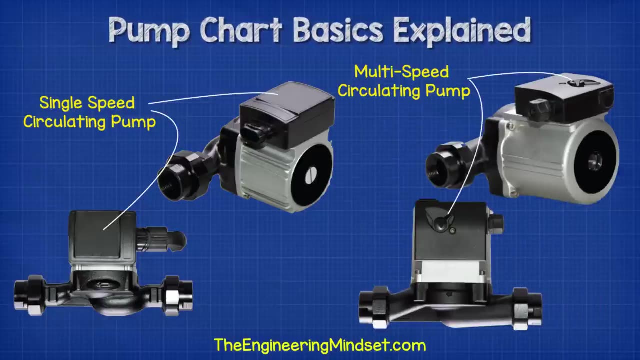 of around 4.5.. 9 feet Multi-speed pumps. Some pumps, such as this one, operate at a fixed speed and therefore have a fixed performance curve, But we can also get multi-speed versions which have the ability to switch between speed settings. 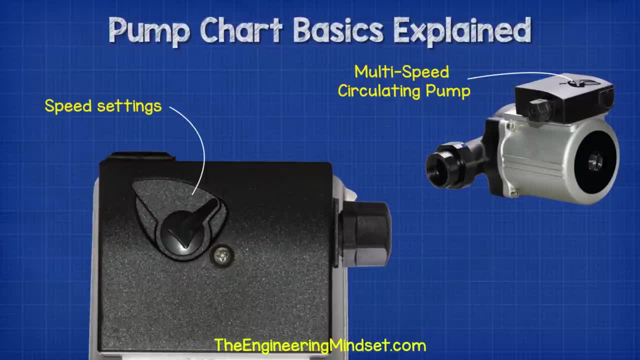 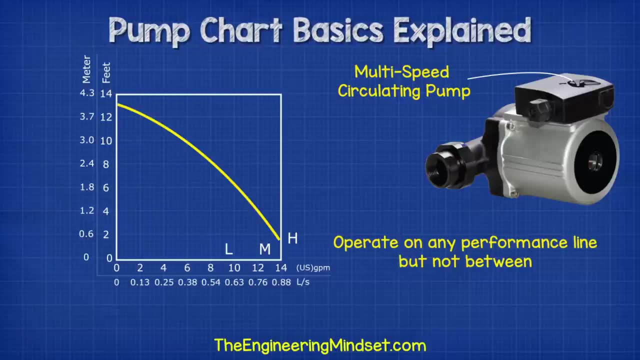 Typically, these come with three different speeds: low, medium and high. These pumps will therefore have a chart with three different profiles plotted on them. We can operate the pump at any of these curves, but not between them. So, for this example, if we wanted six gallons, 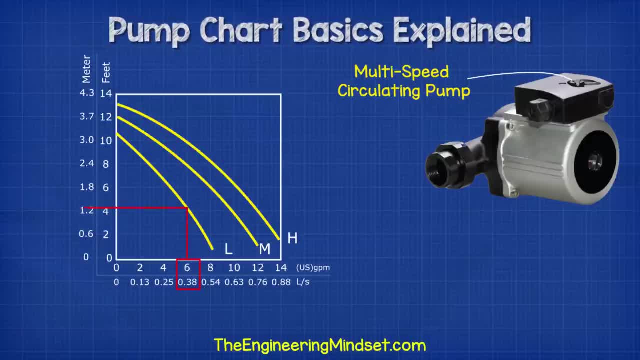 per minute, or 0.3 liters per second. then on setting one, we would get around 4.2 feet of head. On setting two, we would get eight feet And on setting three we would get around 9.8 feet. 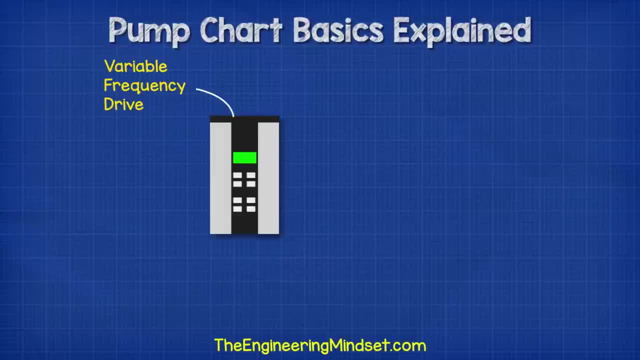 Variable speed or variable frequency drives. Another option we have is to use a variable frequency or otherwise known as a variable speed drive. This basically takes the electrical supply and alters it to reduce the voltage and frequency, which therefore alters the power of the motor and the speed of the pump. 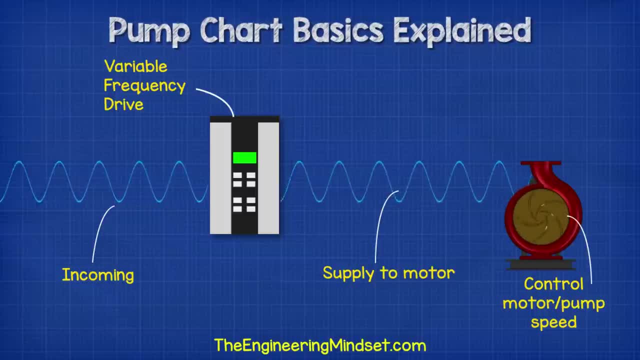 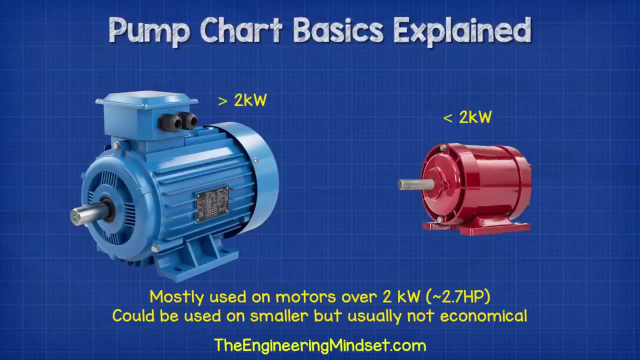 We can increase or decrease the speed via the controller to better improve our pump match and therefore operate nearly anywhere in the region below the curve. These are only really used on larger pumps, typically over two kilowatts in size. They do come pre-installed with new pump motors. 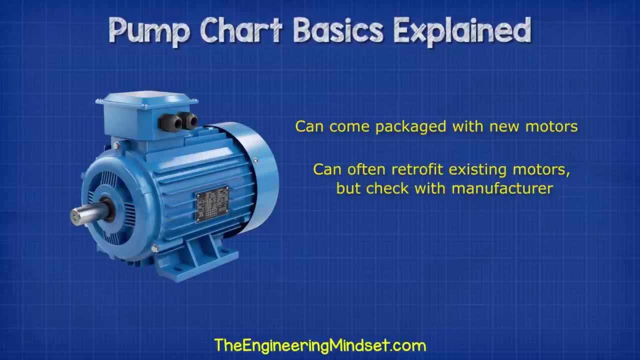 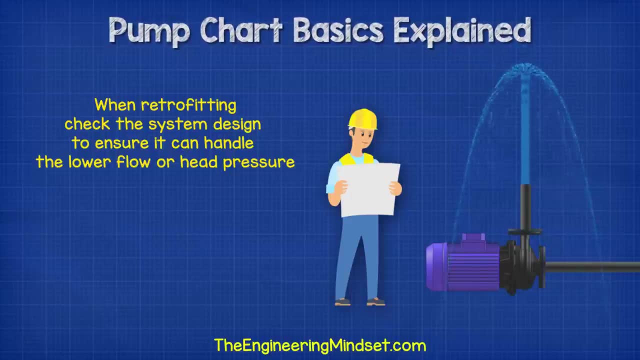 or you can also retrofit existing pumps, But you should check with the manufacturer first to ensure compatibility. Additionally, you must check the system design to ensure it can handle a lower flow rate and head pressure. To obtain the performance details for variable speed pumps. 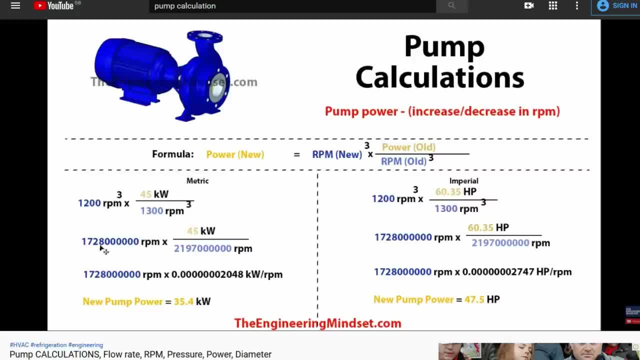 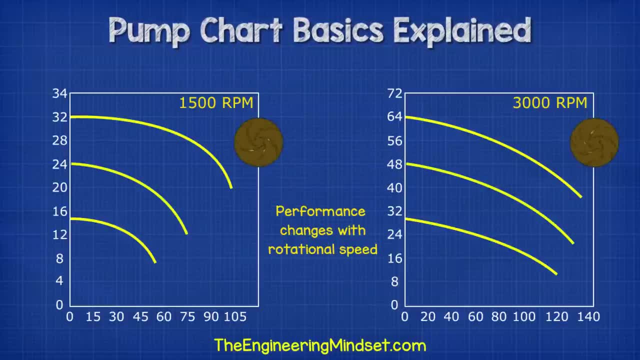 we have to calculate the values using the pump affinity laws. We've covered this previously in worked examples links down below. for that Rotational speed, Some pump manufacturers will provide separate charts for operating the pump at different rotational speeds. We can then compare the performance to get a close match.